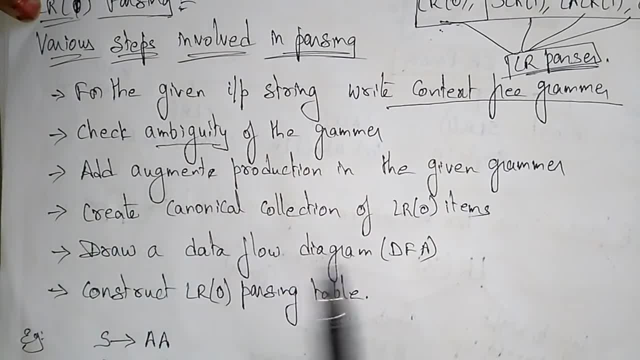 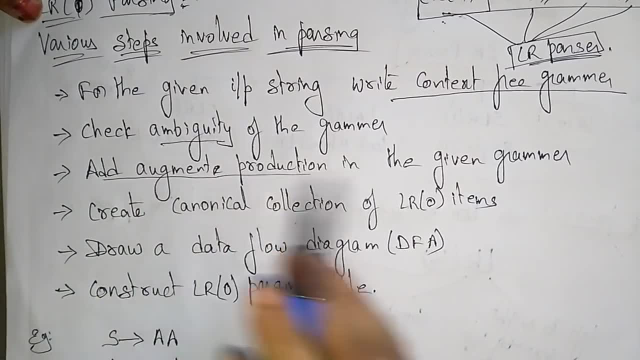 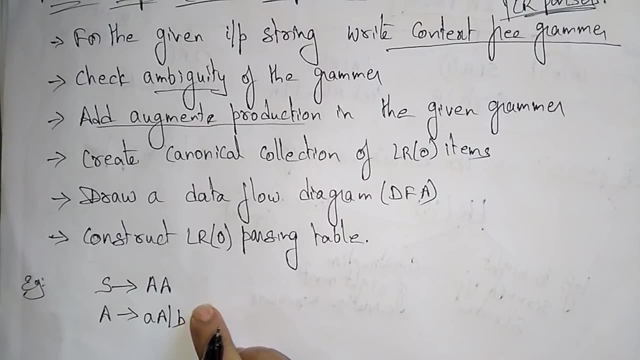 write the context-free grammar and check the ambiguity is there in that grammar. Next add argument production in the given grammar. Argument production means, let's say, G is a grammar. So here you can see, this is a grammar. So if G is a grammar, the argument grammar G will be generated. 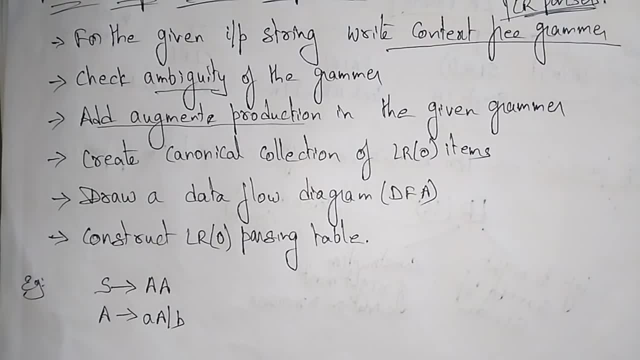 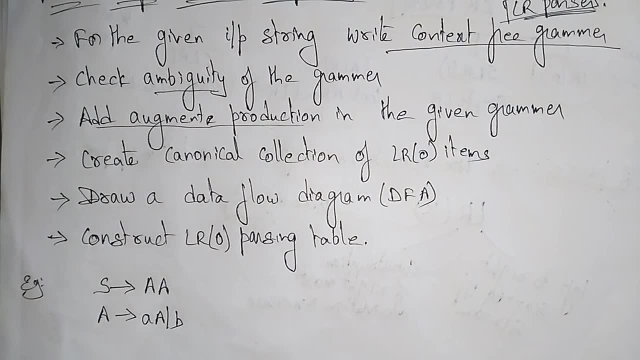 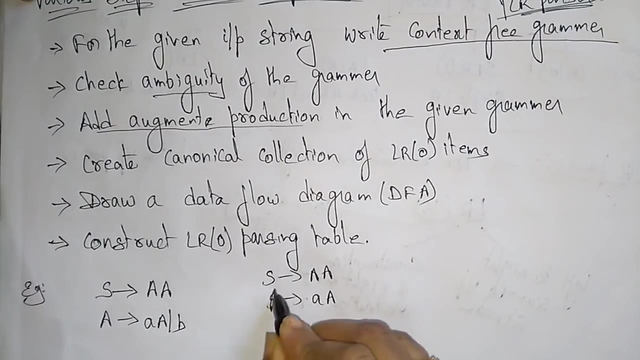 if we add one more production in the given grammar. So this: here you are having 1,, 2, 3.. Three productions are there. Okay, so that means S tends to AAA, S tends to A. sorry, A determines AA and A produces B. 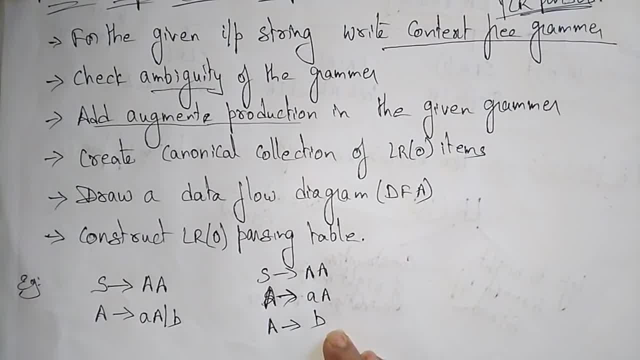 Now there are three productions. Then argument grammar means let's state: G will be generated if. if we add one more production in the given grammar G, It helps. the parser means: I want to add one more grammar here. If I add one more grammar, that is one more production. let's take S. 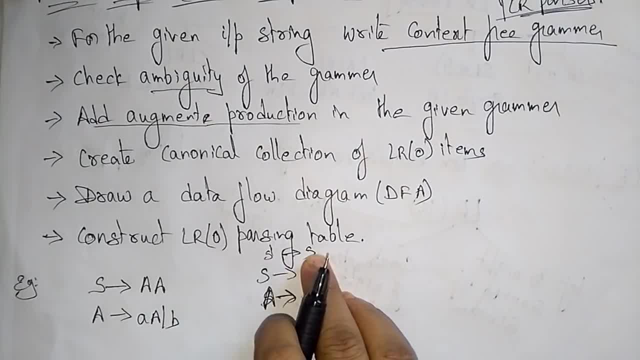 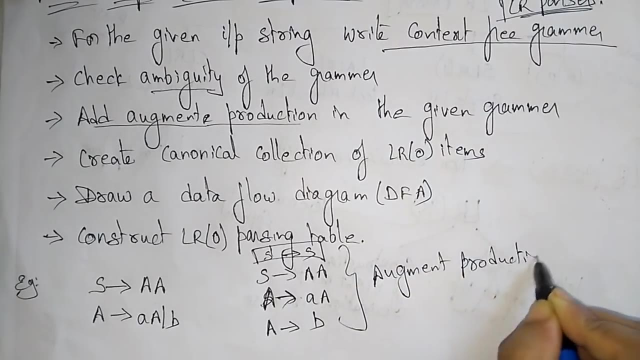 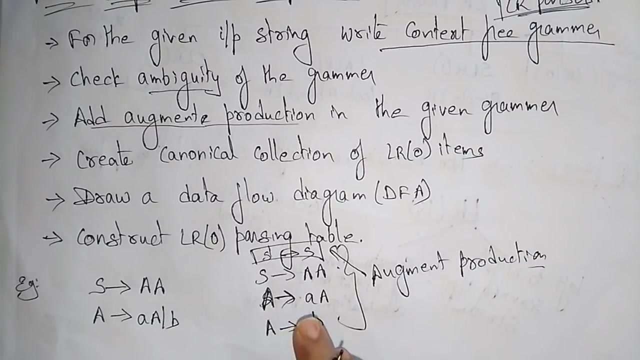 desh ten determines S. Okay, so I just added 1 more production. So then, what is the use of this production? whenever you add 1 more production, you call it as an augment grammar, augment production. so this thing is the augment production. so why i am adding the augment production in the given grammar? so if you do this, 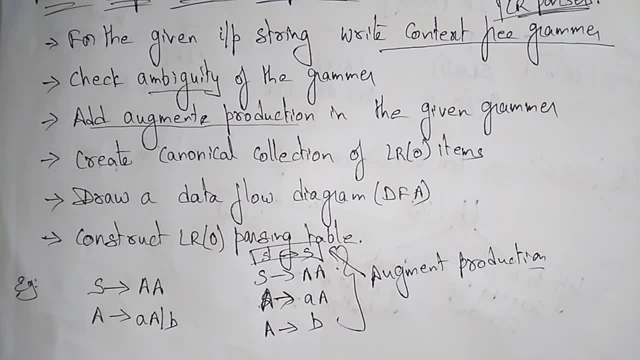 it helps the parser to identify. it helps the parser okay, that is the lr0 parser. it helps the lr0 parser to identify when to stop the parsing and announcing the acceptance of input. so if you use this augment grammar, augment production, this augment production is going to help you to identify when to stop the parser okay, and announce acceptance of a string. 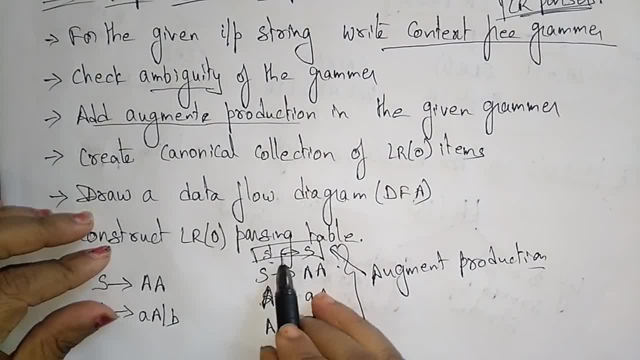 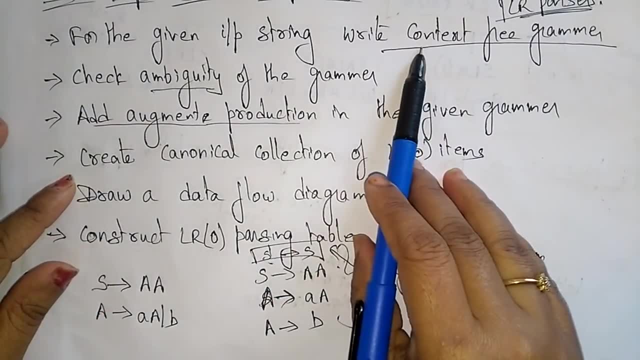 okay, so that is just simply add one more production. s dash tends to s s dash determines s. okay, after adding the first check, write context-free grammar and check the ambiguity. next, add augmented production. okay, after adding the first check, write context-free grammar. okay, after adding the first check, write context-free grammar. 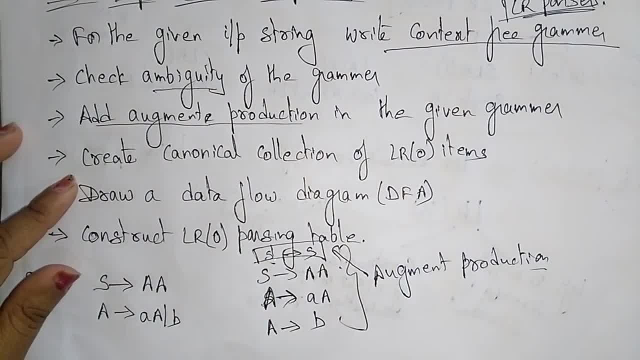 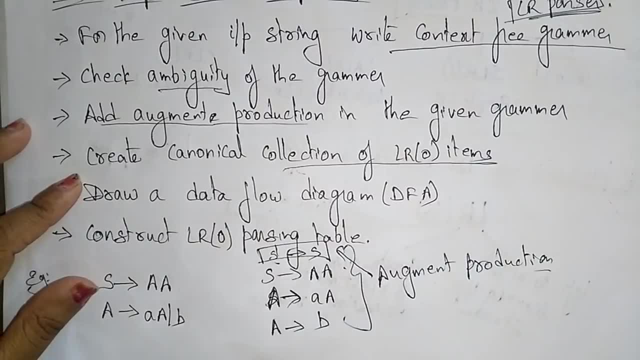 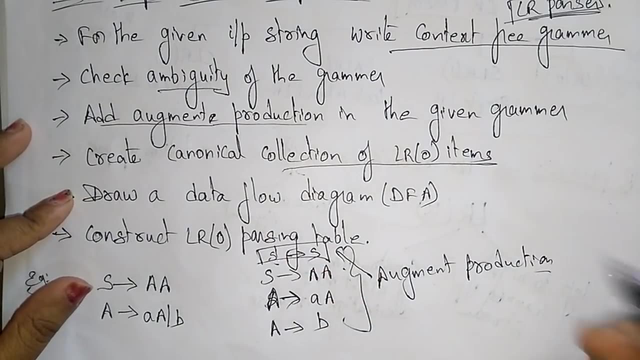 create a canonical collection of lr0 items. i said in the previous video. okay, first thing is you need to create a collection of canonical lr0 items. lr0 items you need to find out. okay, so, after finding out the canonical collection of lr0 items and draw a data flow diagram for that items, 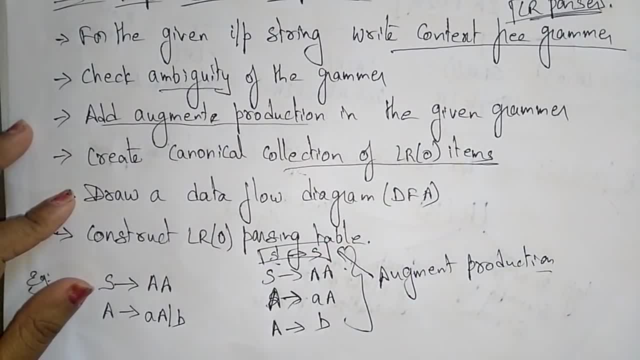 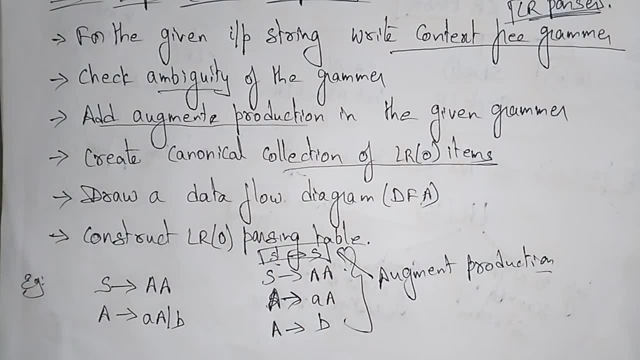 so, whatever the items that you have taken for the items, you need to draw the data flow diagrams and finally construct the parsing table. okay, so after constructing the parsing table, still you need to. if you want to parse the input string by seeing the parsing table, you just need to. 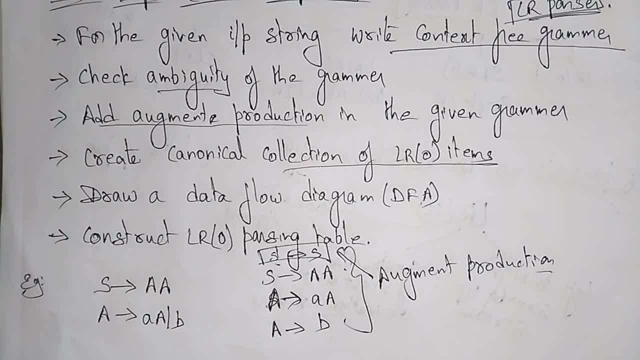 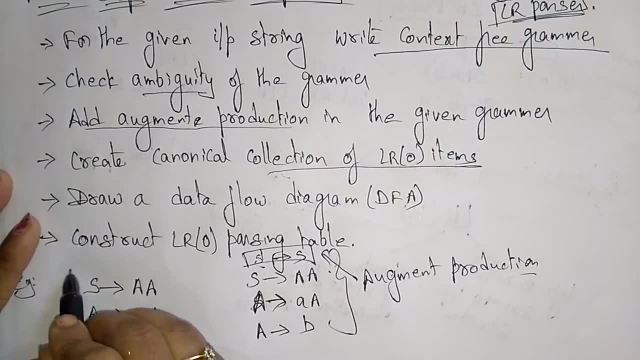 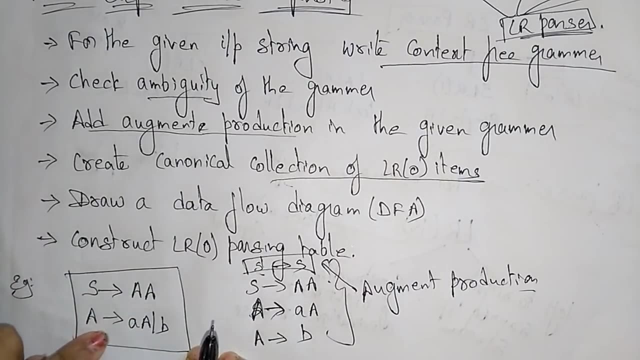 construct the input string. that is a stack implementation. finally, the tree diagram. okay, so let's take this example to construct the lr0 parsing. so this is a given grammar: s determines aa and a is determines aa slash b. okay, so this is a context free grammar and here there is no ambiguity, is there? now i need to. 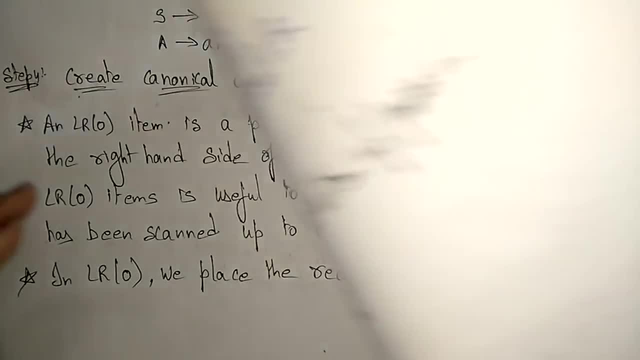 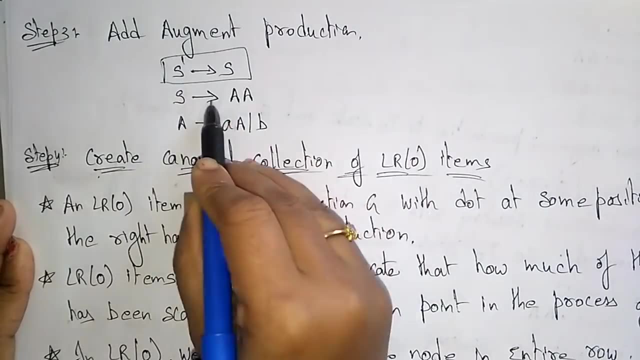 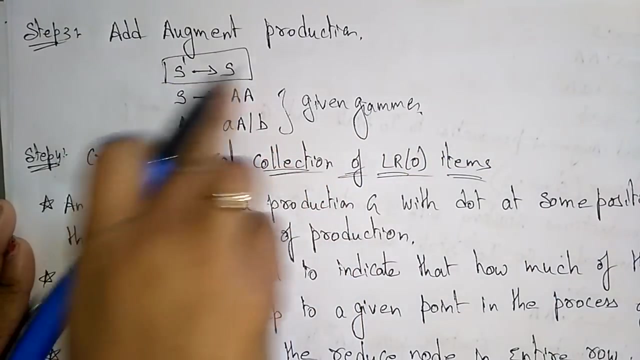 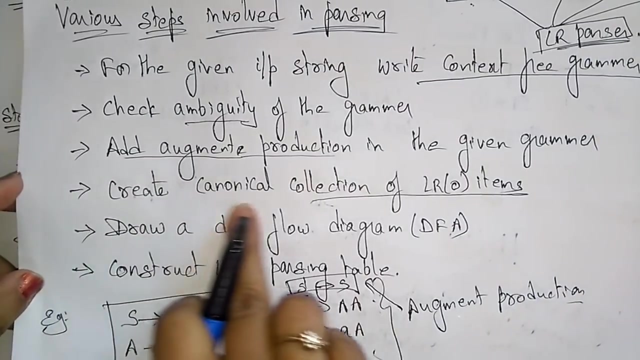 add. the third step i need to add is add augmented production. okay, so here i added the argument. production, that is, this, is all extra production, so this is a given grammar, this is the given grammar for this grammar. i added the augmented production. so next, what i had to do? the next step is i had to create a canonical collection of lr0 items. 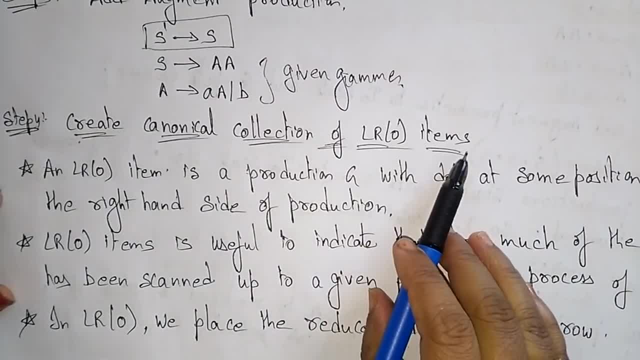 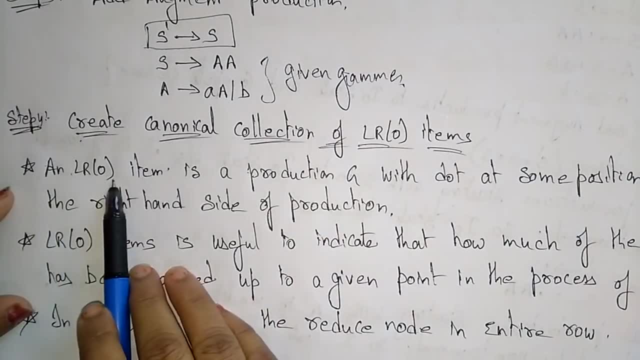 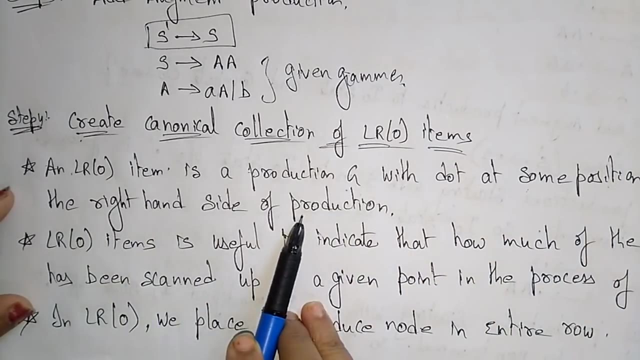 so how you are going to create a canonical collection of lr0 items. an lr0 items is a popular is a production g. sorry, an lr0 items is a production g with the dotted some position on the right hand side of the production. so the canonical collection of items are nothing but any production of lr0 items is a production of lr0 items. 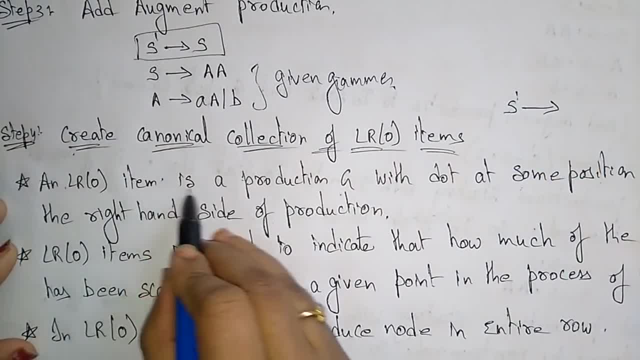 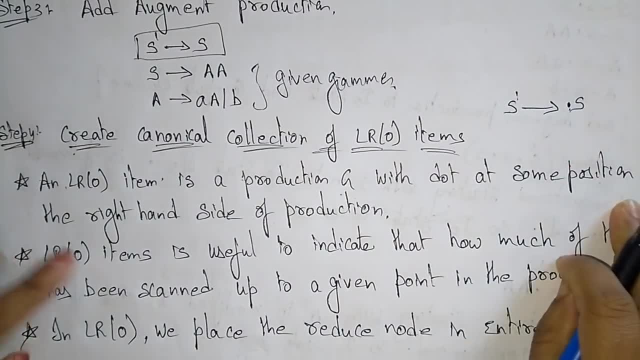 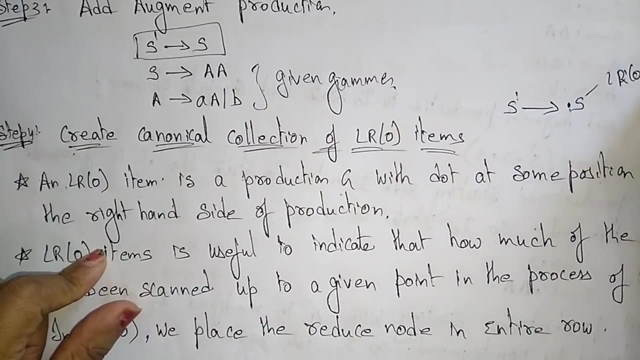 if you are taken. let's take augmented lr0 item is a production g with the dot at some position. so the dot should be at some position on the right hand side of the production. so here dot should be there. then this is lr0 item, if dot is there. so after dot the right hand should be. 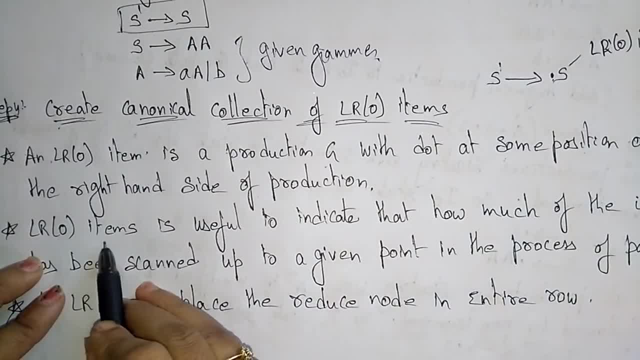 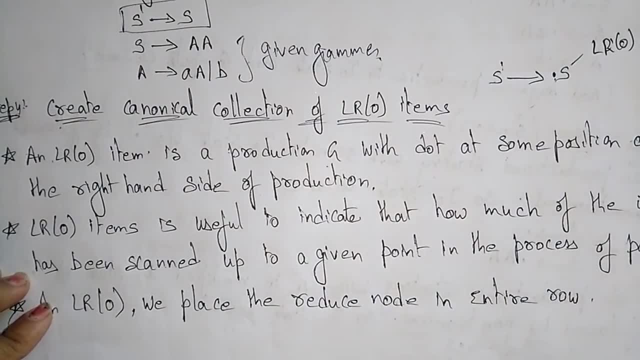 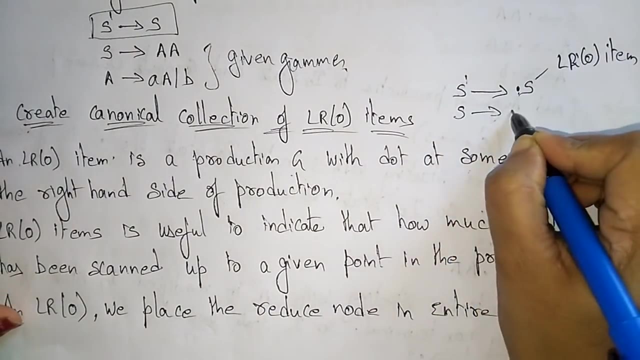 a non-terminal and see the second one, lr0 items is useful to indicate that how much of the input has been scanned up to a given point in the process of passing you, everyone will get a doubt. why are you? why we are using a lot zero items, just placing a dot in the 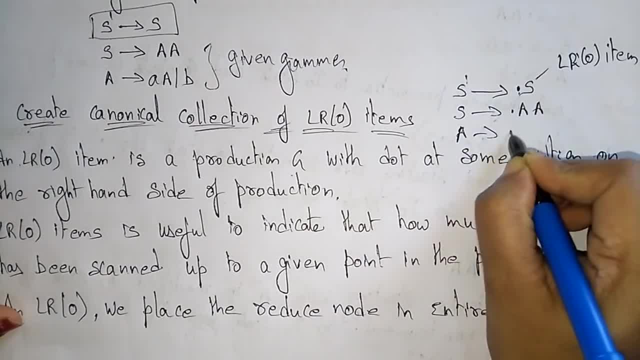 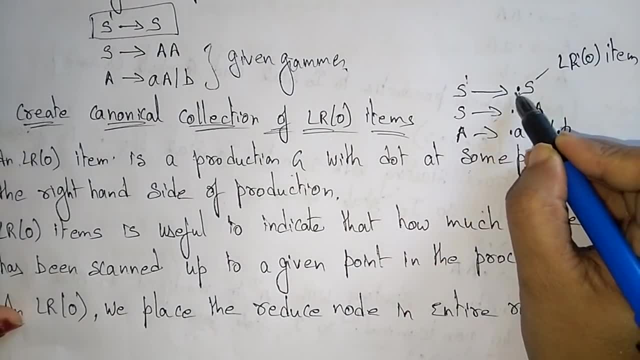 right hand side protection. just, i am placing a dot in the right hand side protection, so these are all becomes the so whenever a dot is there. so after a dot, if the terminal symbol is there, means a closure of s. this you call it as a closure. the closure of s has to be. 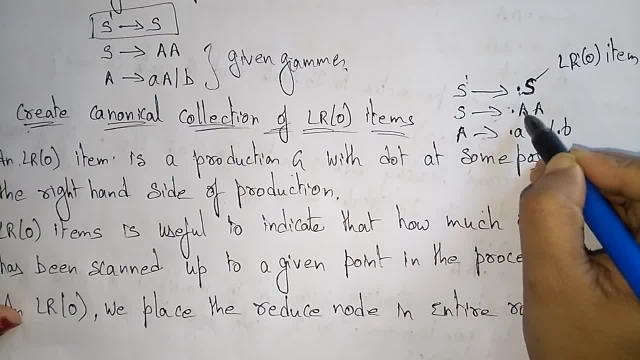 general. so generator, again s tends to dot a, a. so again in after the dot a non-terminal is there, then you need to find the closure of, you need to expand the complete productions of that closure. so dot a means again a tends to dot a a slash dot b, but after the dot there is only the terminal. 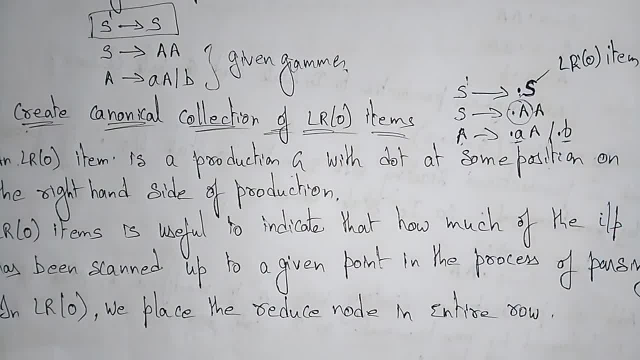 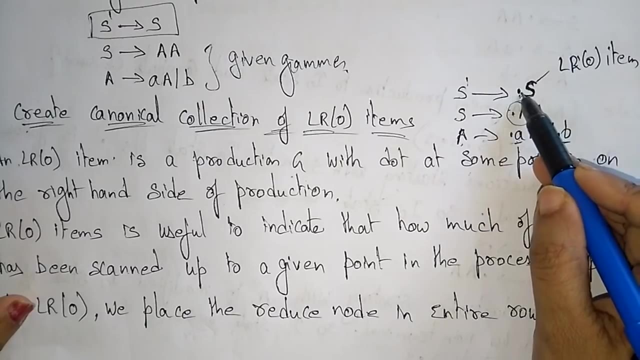 symbols are there. there is no non-terminal. okay then you no need to extend the productions, you no need to write the productions, because dot a terminals has have no productions, only the non-terminals will have the production. so, whatever the productions that are produced by the that 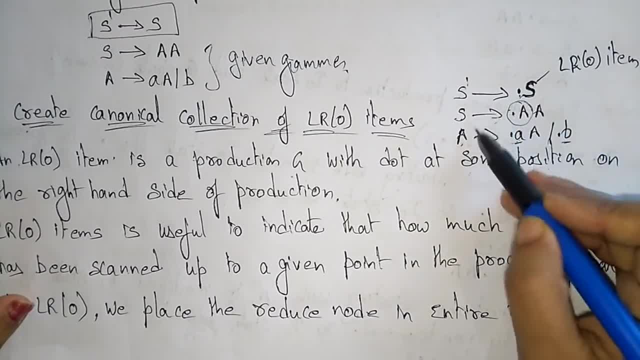 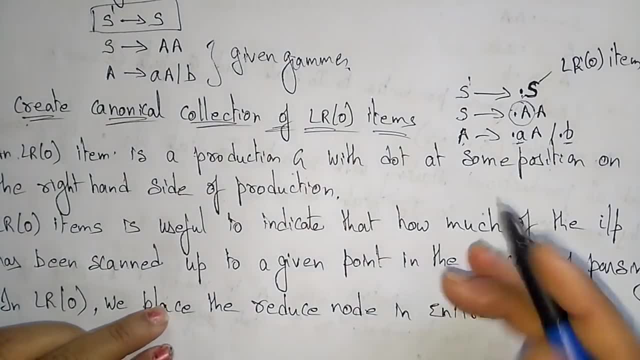 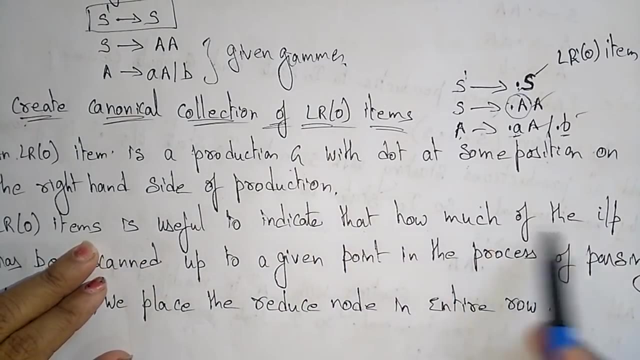 non-terminal. after the dot for those productions you need to write everything dot one. so now see why we are using the dot. so the lr0 item, these are all lr0 items. the lr0 item is useful to indicate that, that how much of the input has been scanned. so for each and every step the scan is moving. 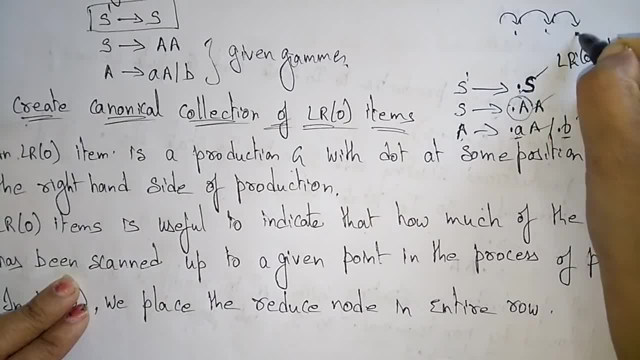 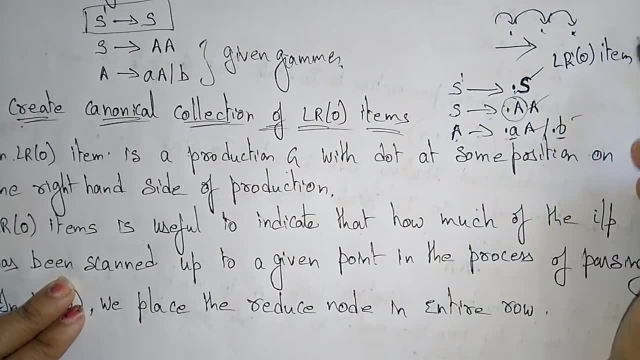 to the right hand side the dot, the scan is doing the right hand side, the scan will be moving, so it's rightmost derivative. so whenever here the dot is useful to indicate that how much of the input has been scanned up to a given point in the process of parsing, so in 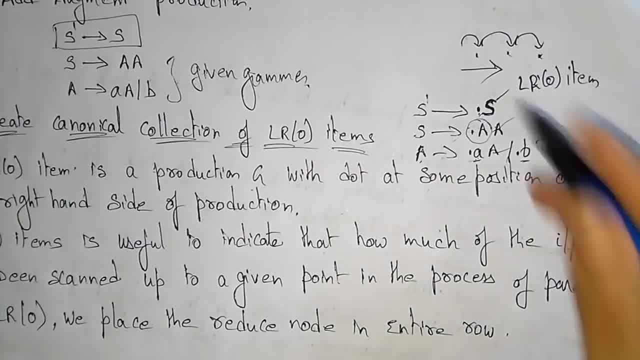 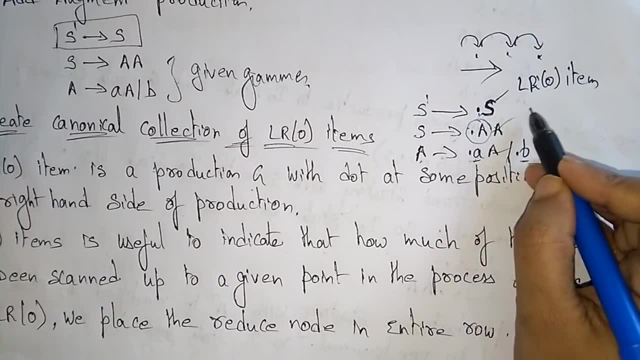 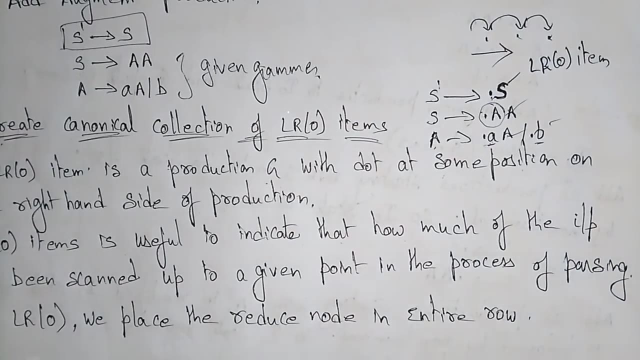 LR0. we place a red juice node in entire row. so whenever, if you reach to the last, if the dot is moved to the rightmost, if there is no terminal or non terminal is there, okay, then you can say it is a. we place a red juice node in entire row. so don't be confused if 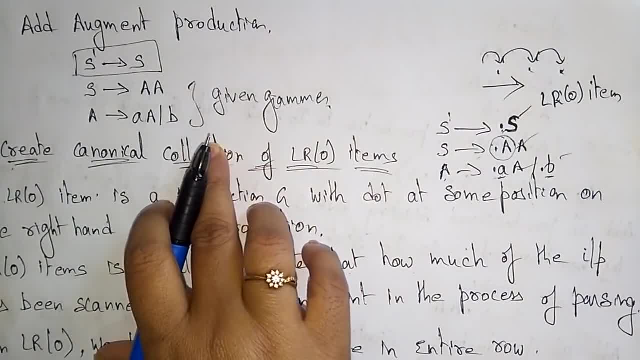 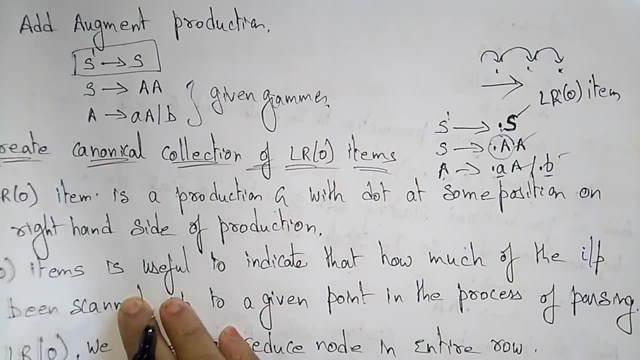 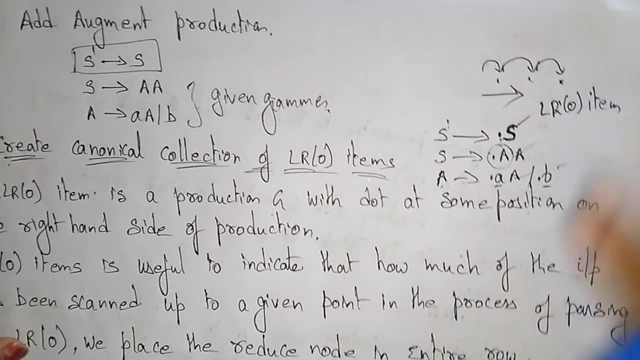 you take the example, so this is the example. whenever you are constructing the drawing the DFD diagram and constructing the table, it will be clear for you: okay, so okay, creating table: canonical collection. so next, what next is I have to draw a data flow diagram. so with 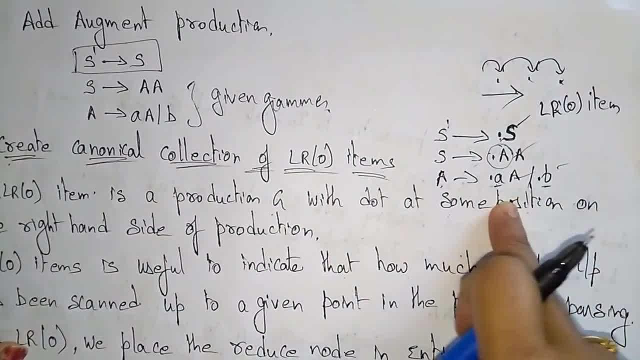 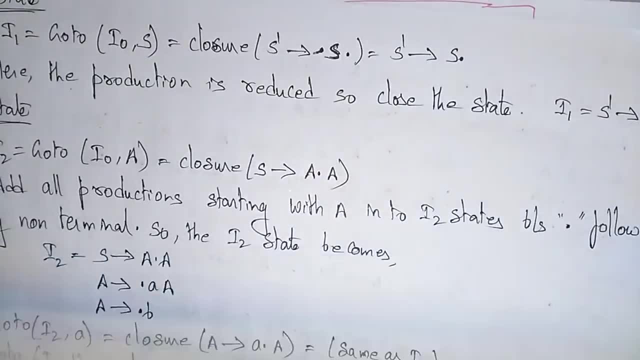 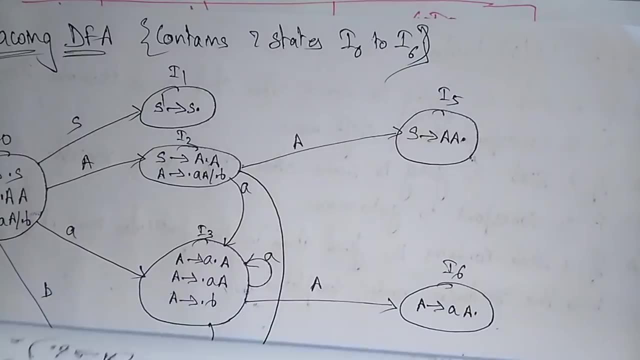 the help of the canonical collection items means the LR0 items. I am going to draw the data flow diagram, DFA diagram. okay, so these are all the steps to follow for each and every state. I have taken I0, I1, I2, different states. now let's see the drawing of canonical by. 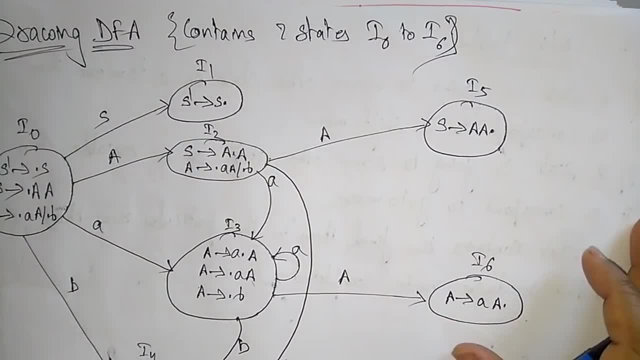 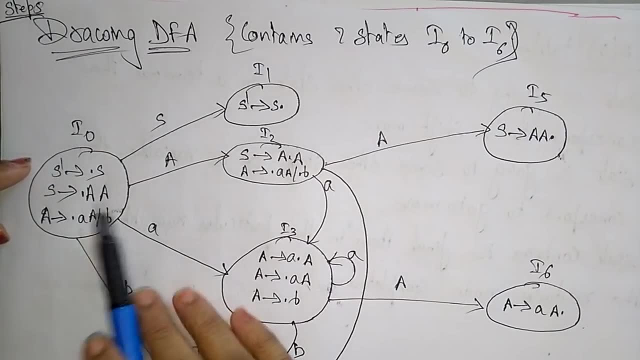 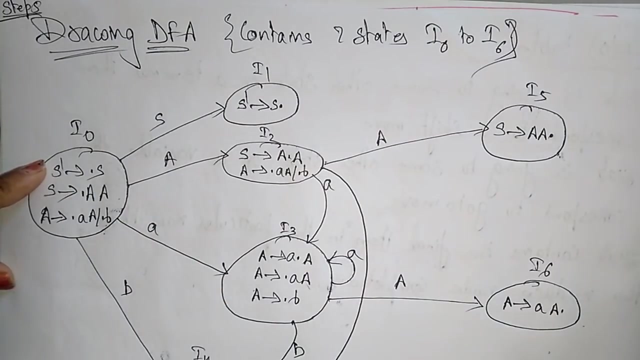 using the data flow diagram: canonical items. let's draw DFA diagram: data flow diagram. so this is the canonical items. LR0 items- canonical collection of LR0 items. s dash determines dot s. s determines dot a- a and it determines dot a- a slash dot b. okay, so this state, you call it as I0. let me take the pan. 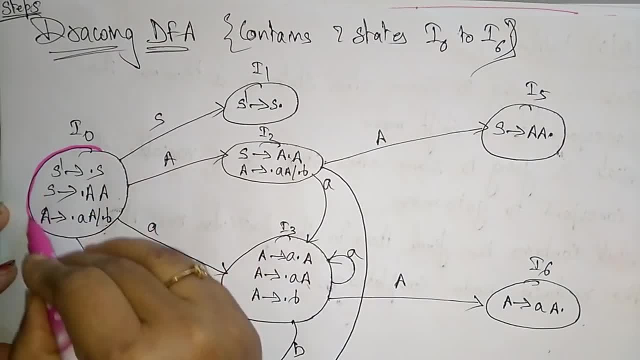 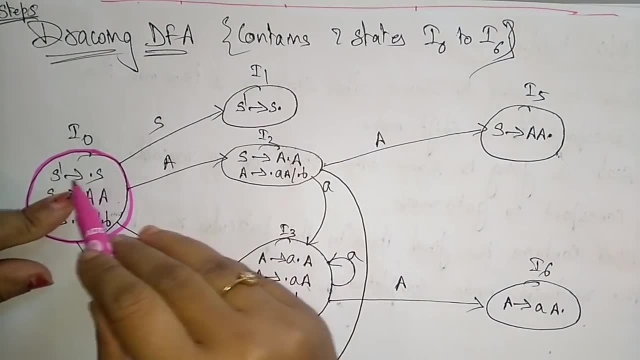 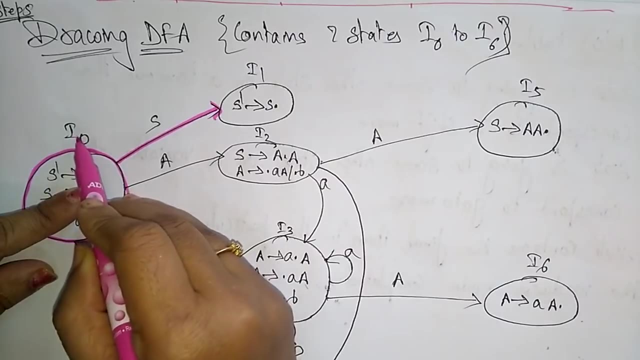 this state, you call it as I0. okay, now let's take first one s determines dot s. so, going on, s I'm moving from state 0 to state 1, that is a I1. so whenever there is a dot here in the right hand side here, you just move the dot to. 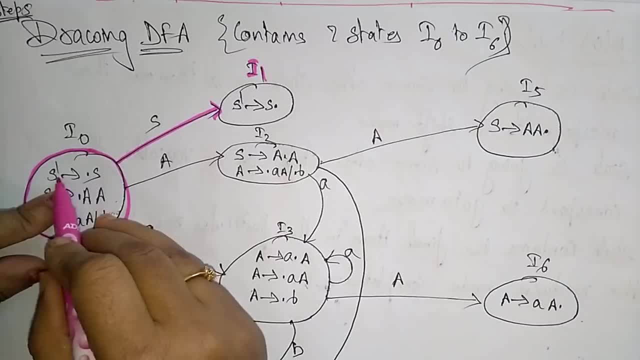 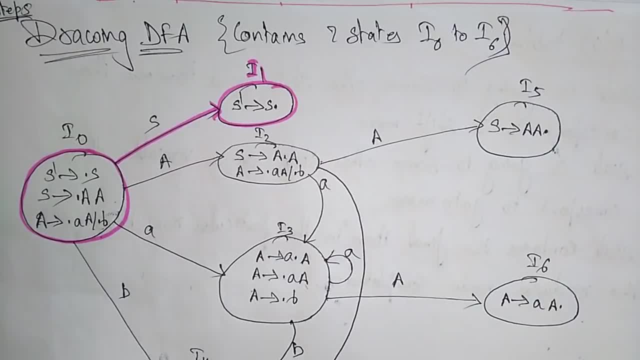 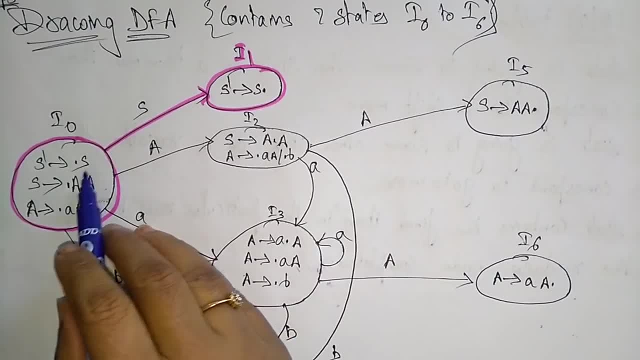 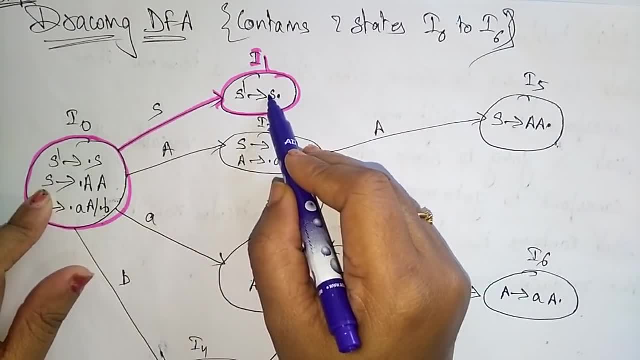 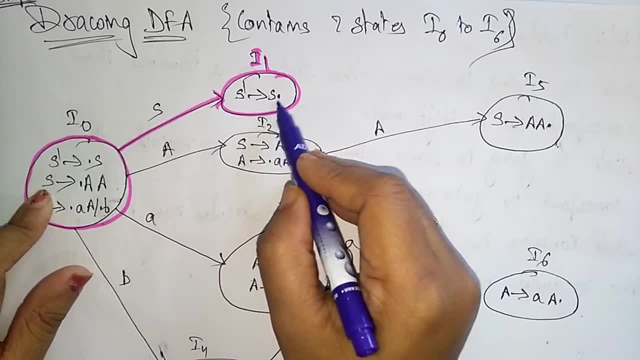 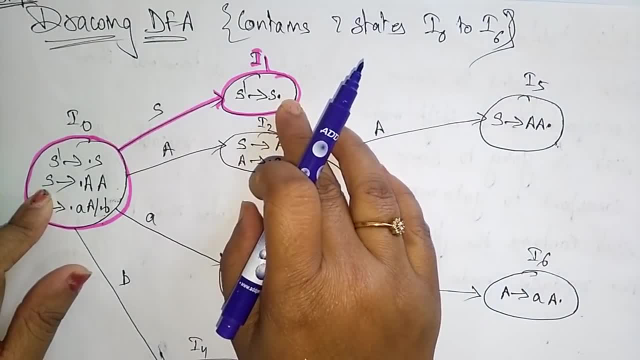 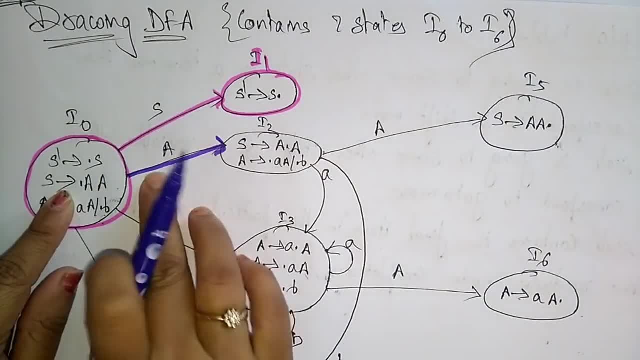 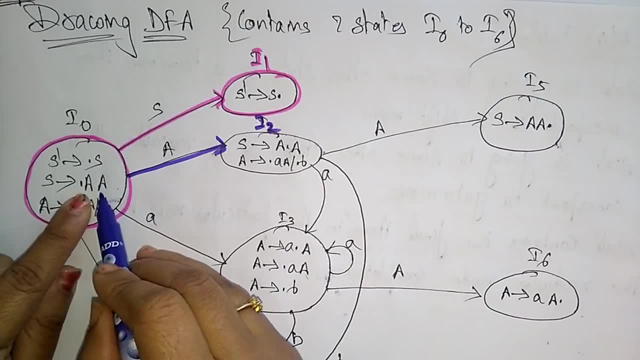 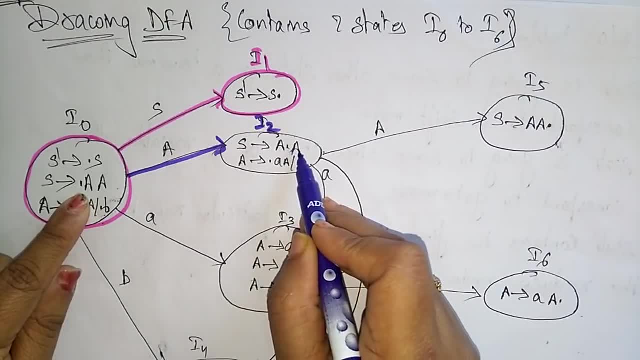 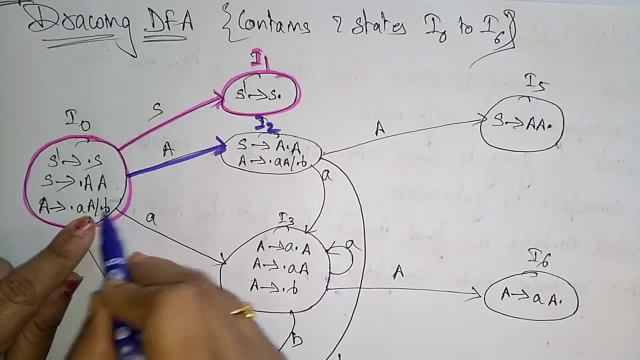 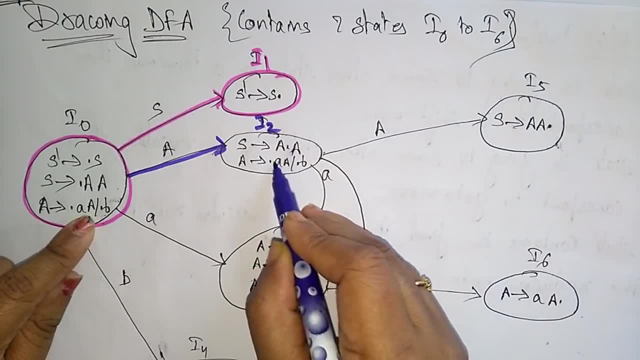 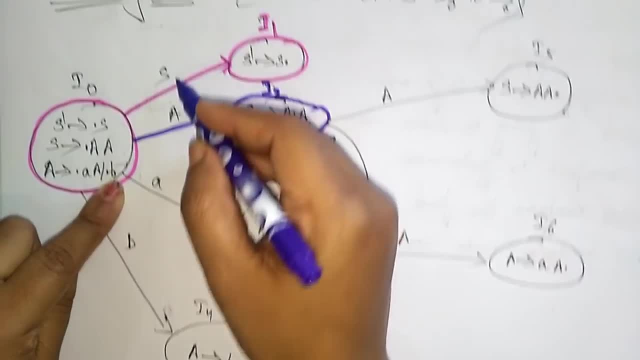 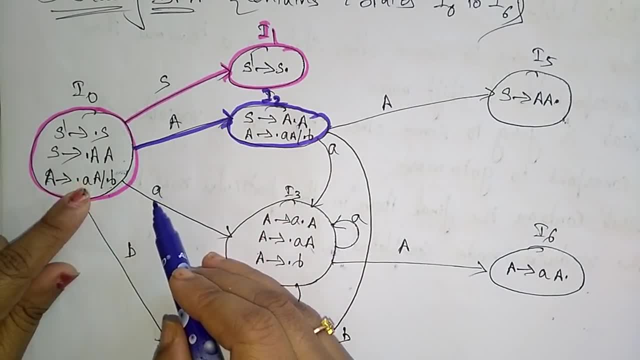 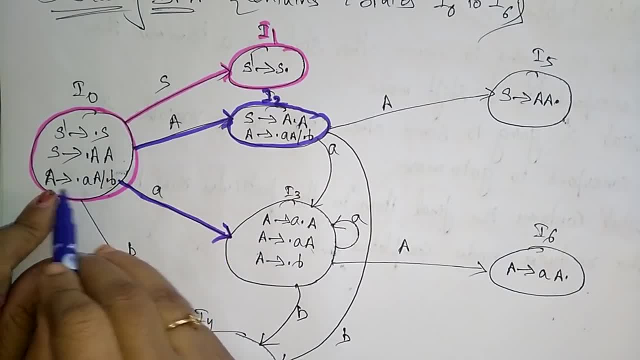 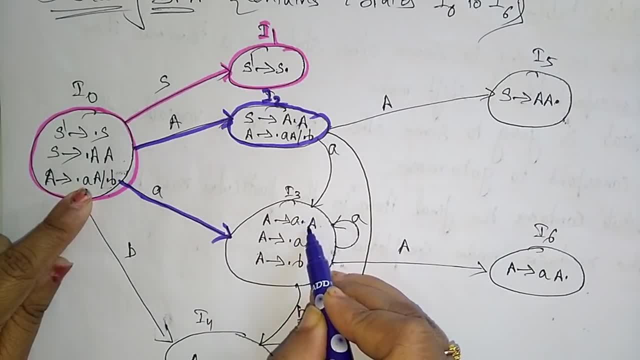 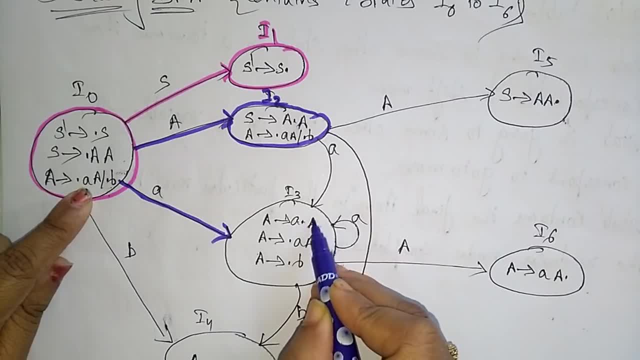 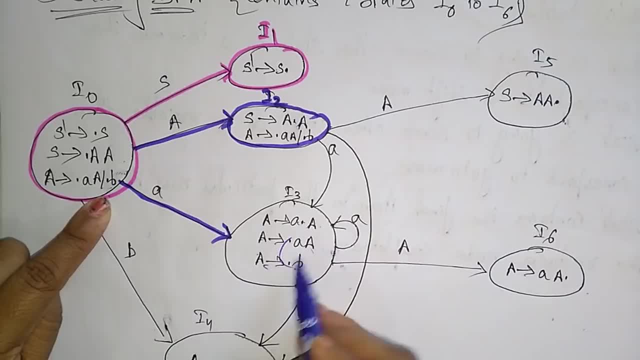 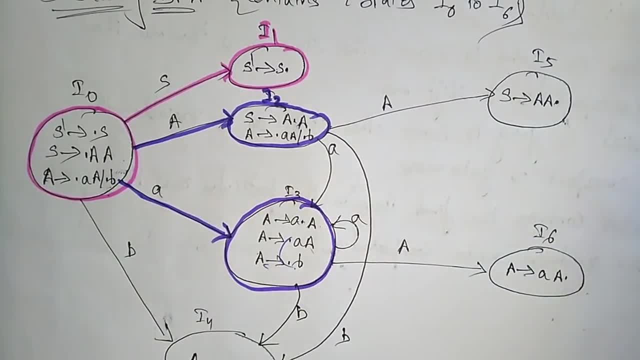 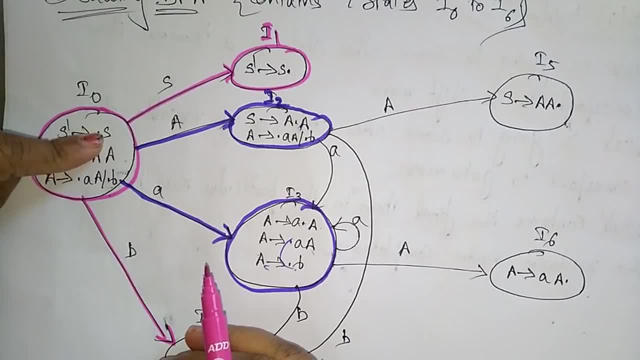 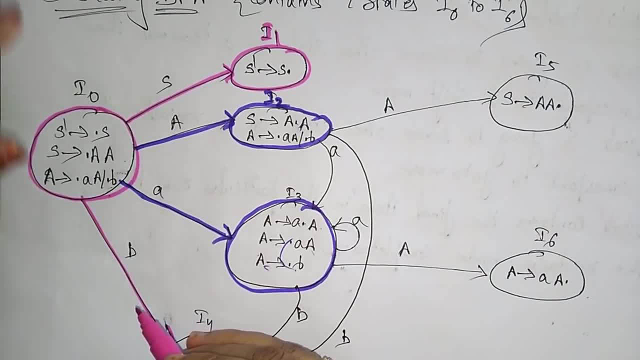 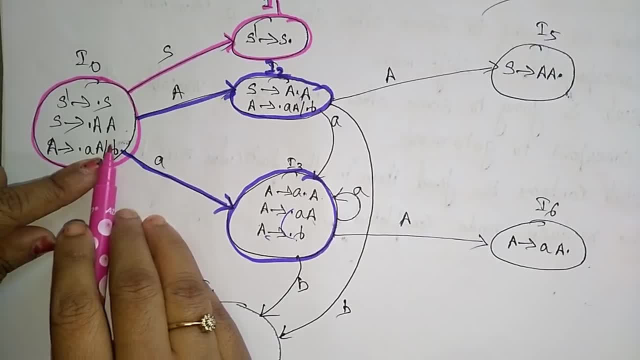 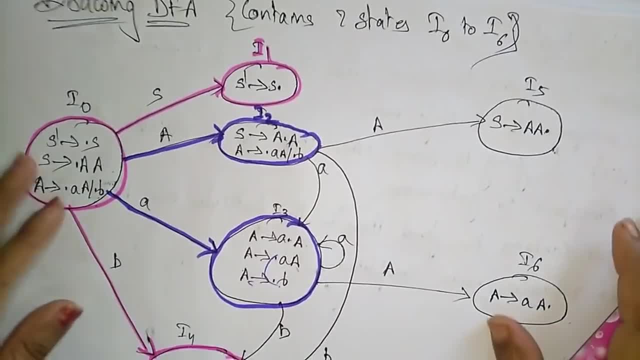 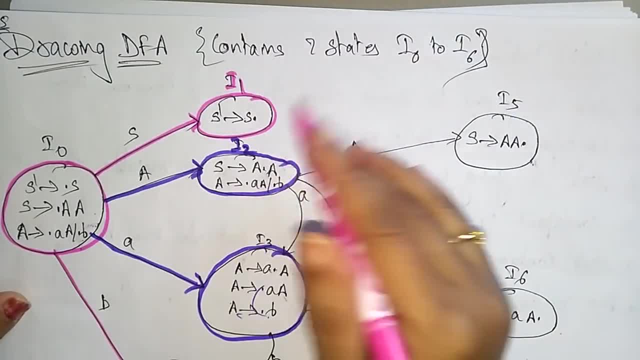 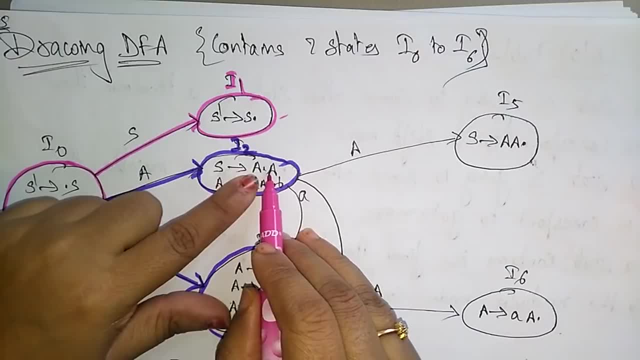 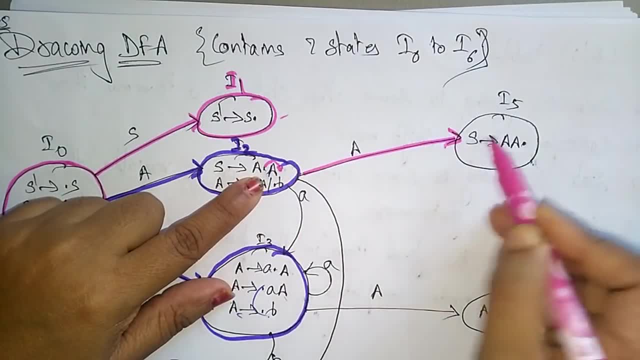 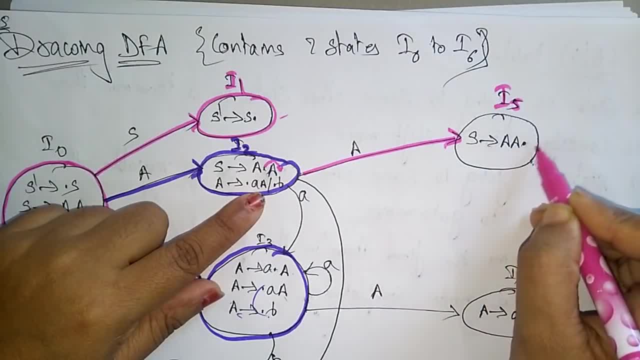 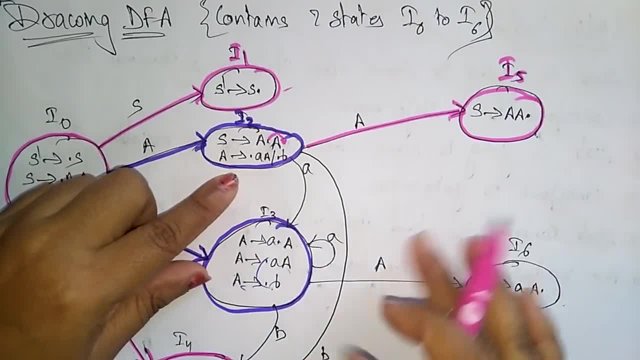 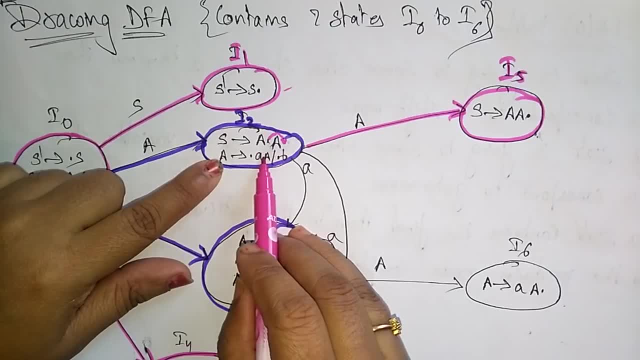 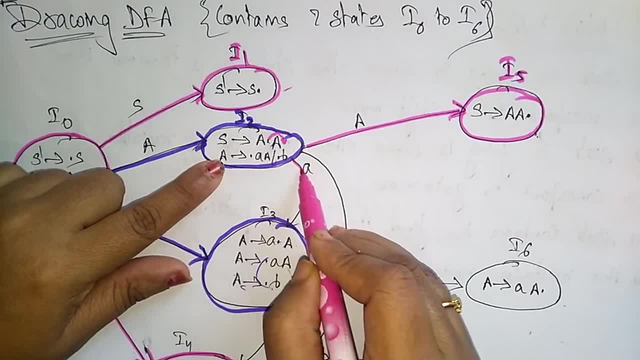 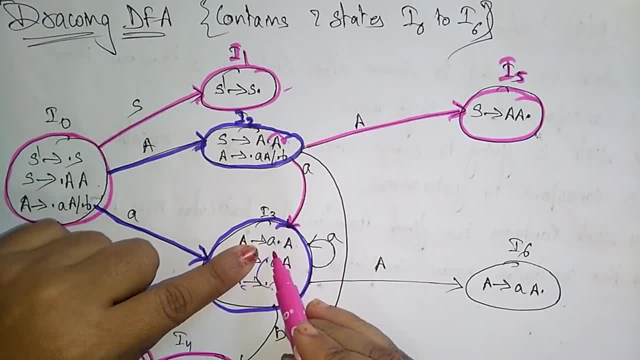 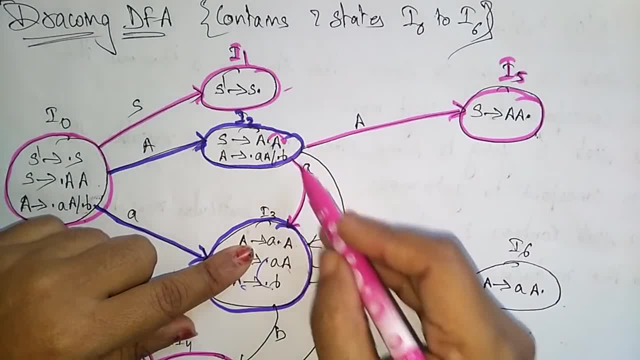 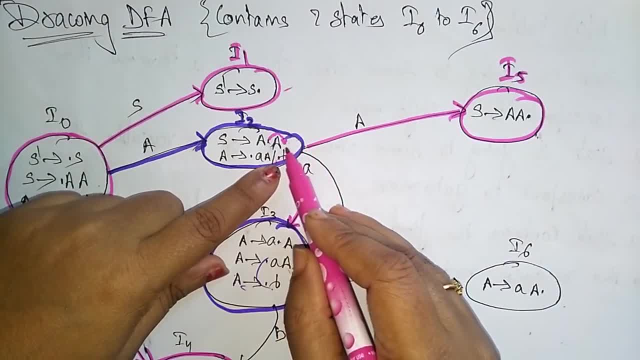 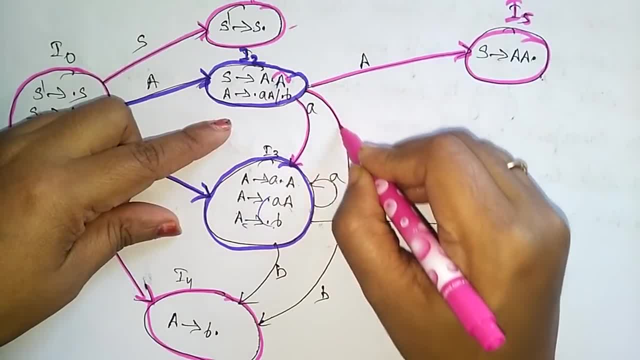 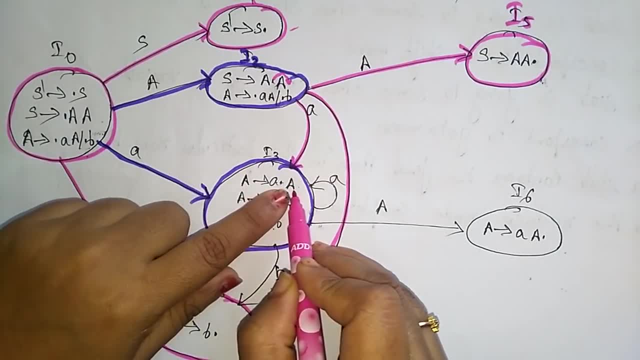 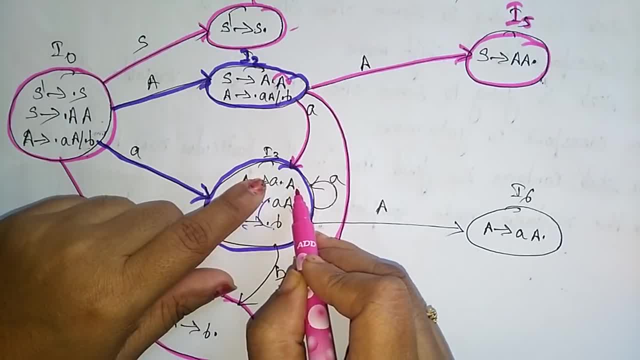 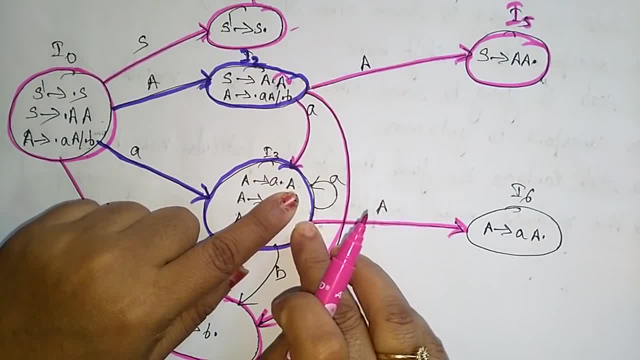 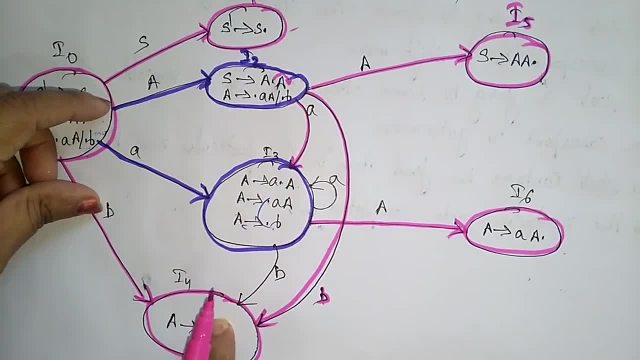 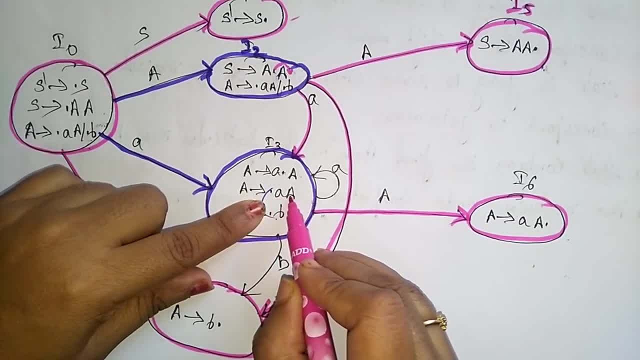 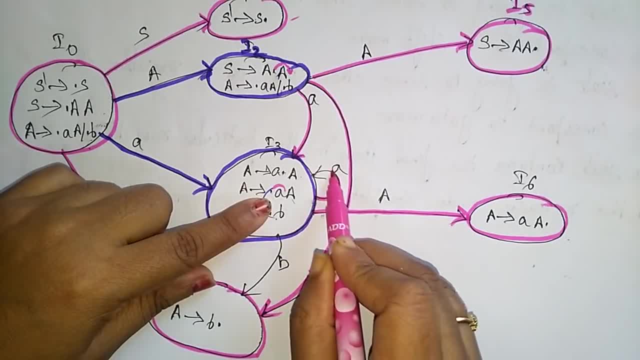 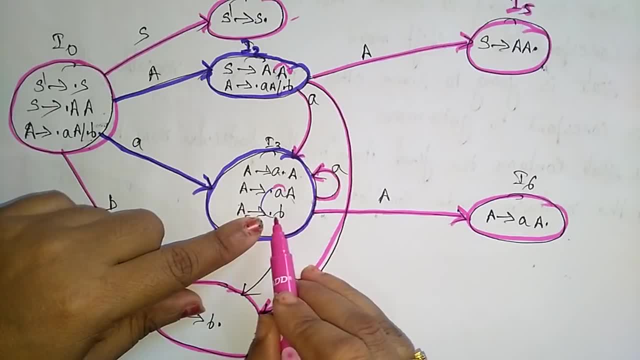 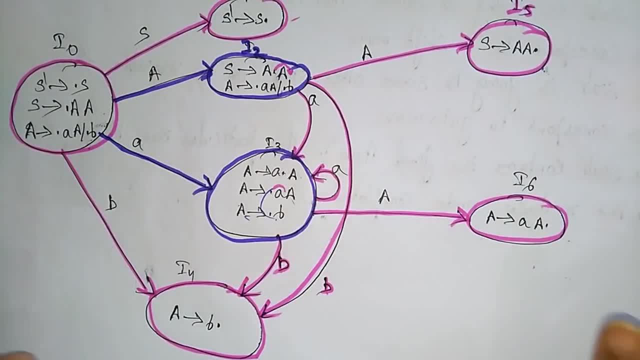 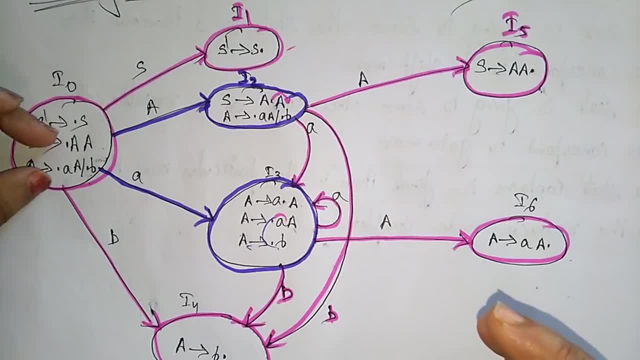 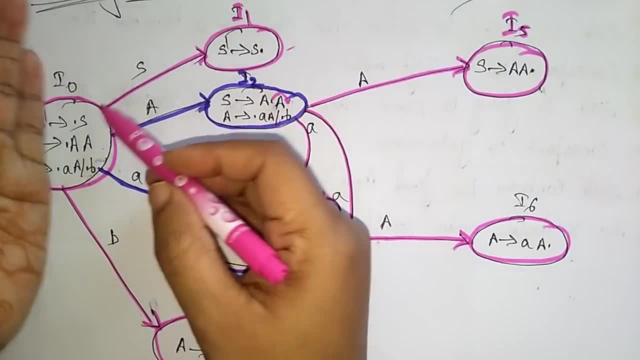 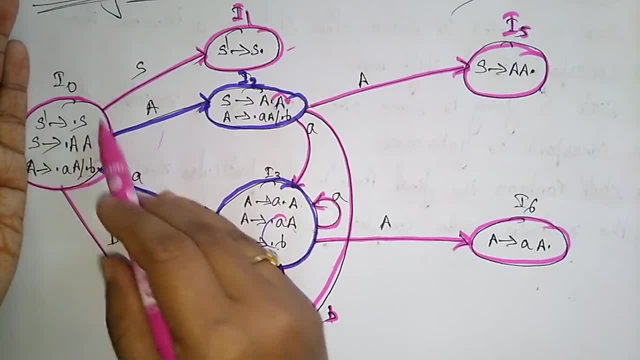 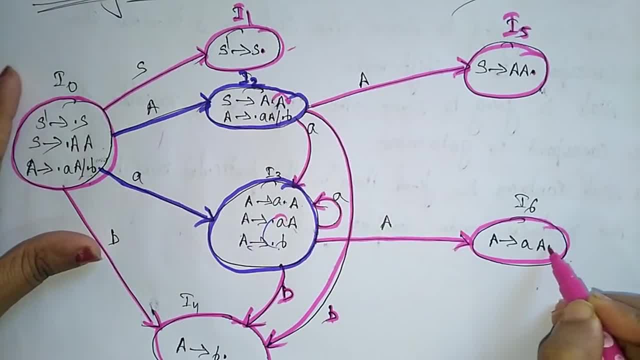 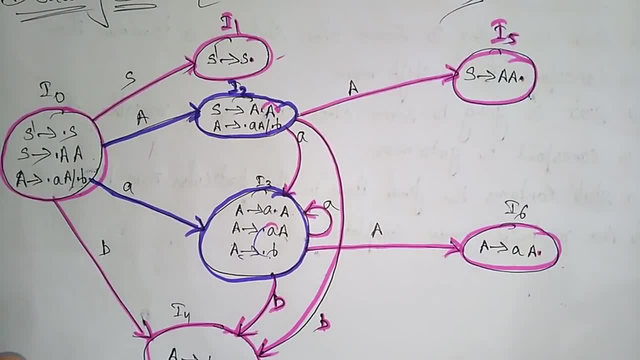 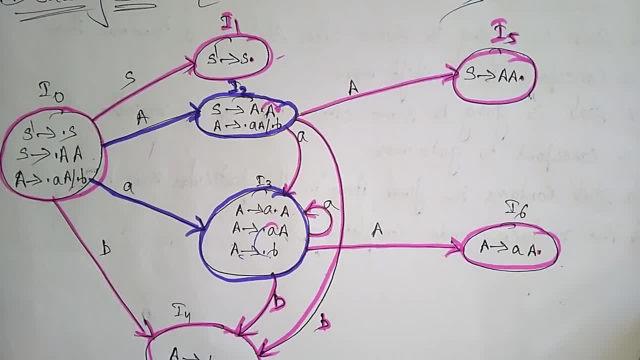